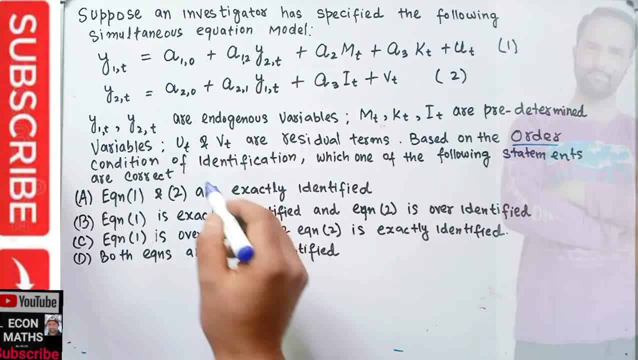 So, based on the order condition of identification, which one of the following statement is correct, We have to see actually which of these equations are either exactly identified, or identified, or under identified. Okay, So for that we use the order condition. Order condition is simple. So order condition tells us: let me write it here first. Order condition tells us: let us say we write k. 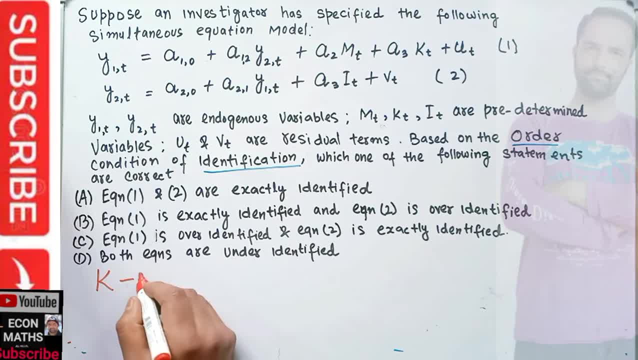 k, k minus m, If k minus m is less than g minus 1.. Okay, In that case we say: the particular equation is what we call unidentified. Unidentified. Okay, But what are these k's, m's and g's? Simply, 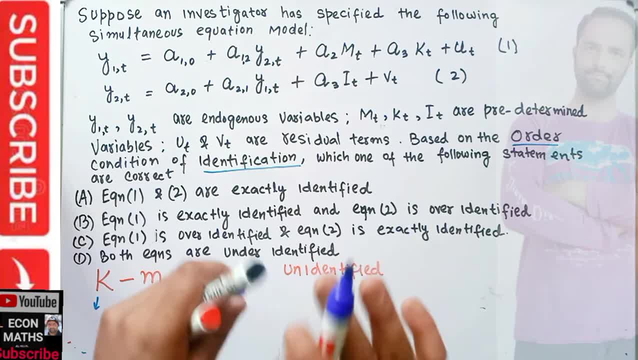 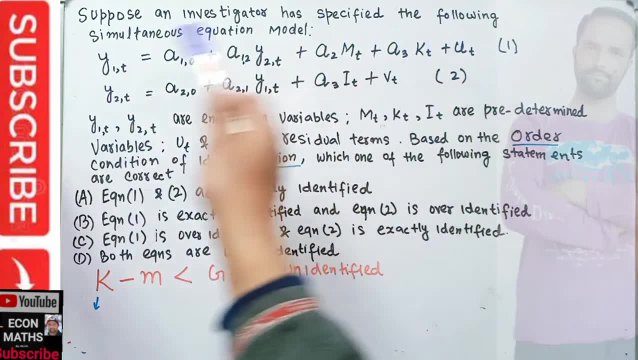 what do these k's denotes? Are they any derivatives or do you have condition in your system like a whole largerłyde or your system itself or any other things? So once I have teen surveyants list, I luckily combine t and v and I d mi over different four subset. 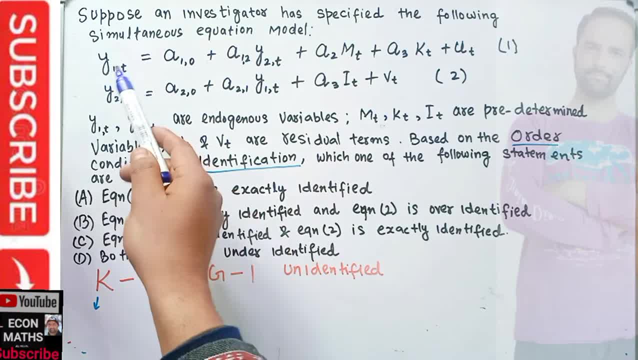 What do find out? this k denotes is the total number of variables, whether they are endogenous or predeterminate variables, in our entire model. Okay, So k denotes the total number of variables in our model. so how many variables we have in this model? 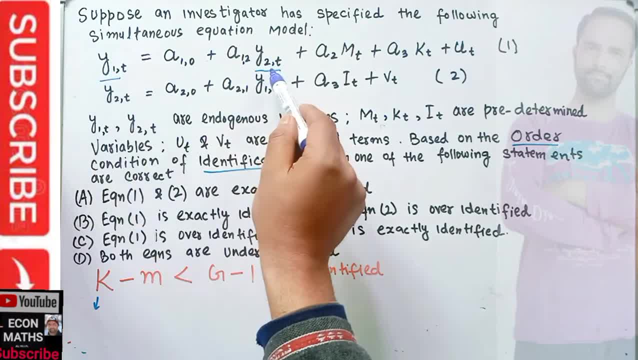 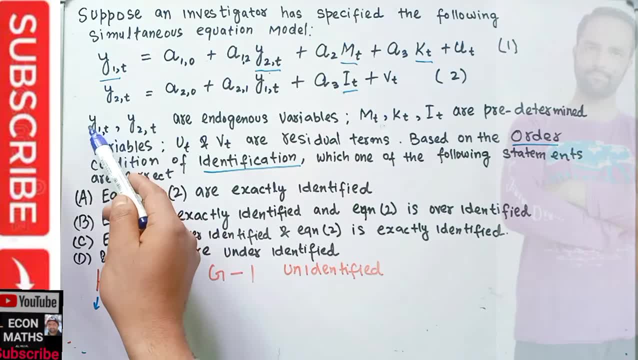 Let us see. so we have one. This is also our 51 2030 Lebanon plan at mmn is also first variable, second variable, third variable variable and fifth variable because we have y1 t, y2 t are the endogenous. 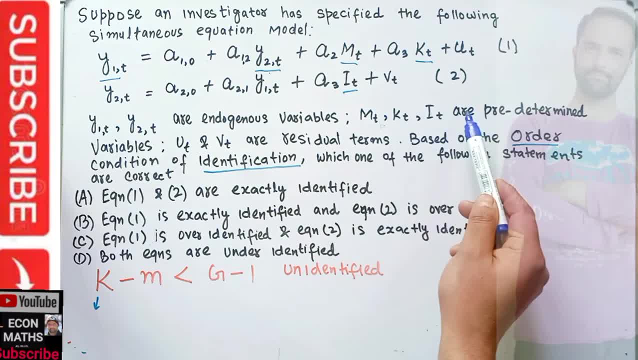 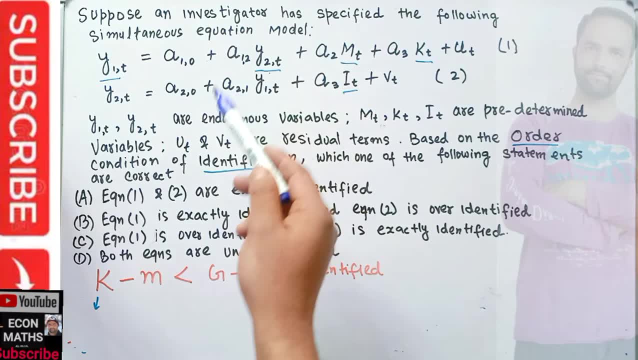 endogenous variables- mt, kt, and it are the exogenous variables. so we have one, two, three, four, five. therefore we have total for you variables in our entire model. this, a a1 not- is not an endogenous or exogenous variable. these are the constant terms. similarly, UT and VT are the residual terms. they are not either. 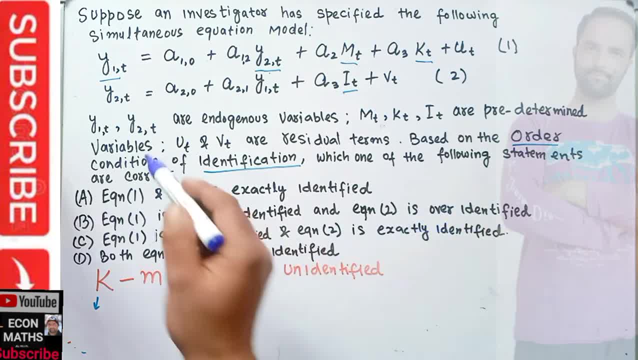 the endogenous or exogenous variables. okay, so total number of endogenous variable is one, two. exogenous variables are one, two, three. so total number of variables in our model are for you, so the value of K is for you, so we have for you. minus M denotes the number of variables in a particular equation. okay, 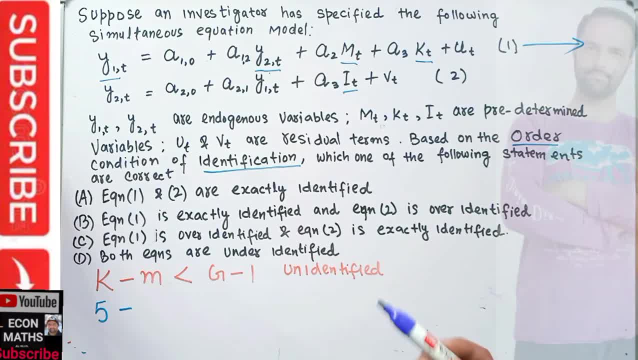 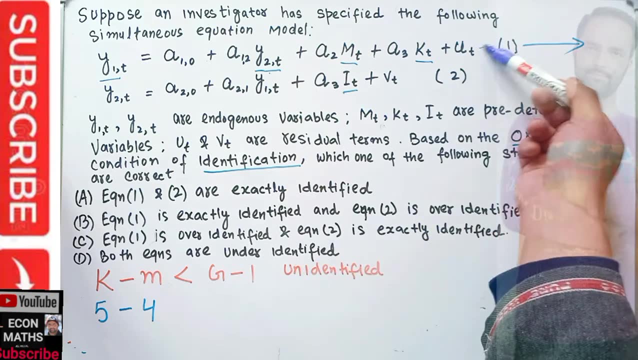 if we take this first equation, let us see how many variables are there. we have one variable, two, two, three, four. we have four variables. that means M is equal to four. okay, and this G denotes the total number of equations. in our model, we have only one equation. 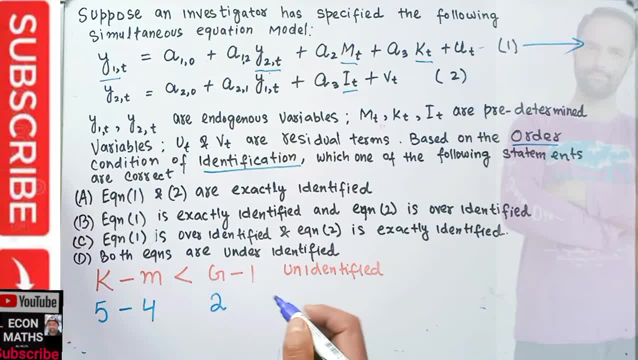 and two equations. okay, so we have two here minus one. okay, so here we can see: five minus four is one, and two minus one is one. here we have: K minus M is equal to G minus one. if this is the case, okay, our case this time would be like this: our K minus M is: 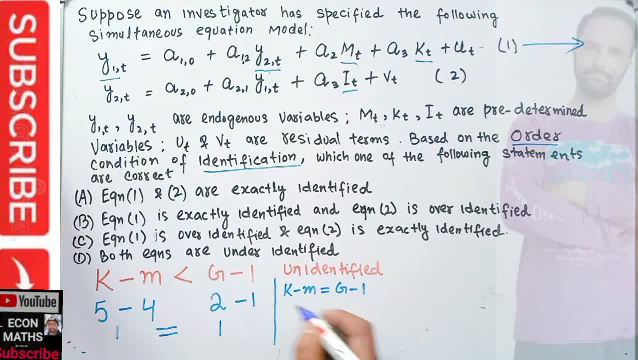 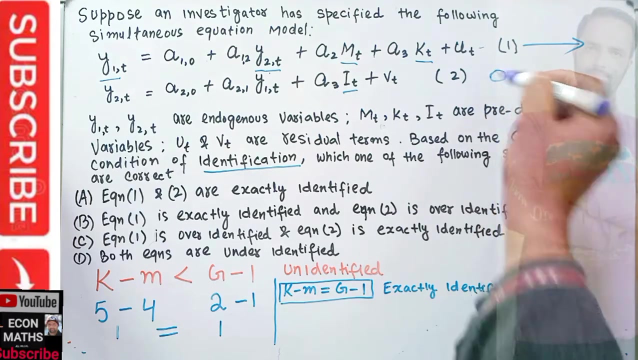 equal to G minus one. if this is the case, we say that the particular equation is exactly exactly identified. okay, that means our first equation is exactly identified. okay now, so if K minus M is less than G minus 1, we have unidentified problem. okay. now talking to second equation, let us say whether the second 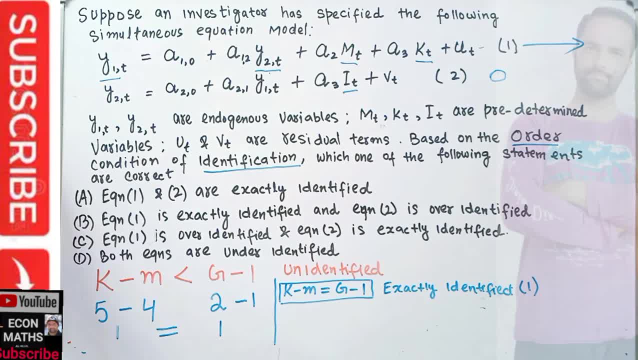 equation is identified or unidentified. for that, using same procedure, K is total number of variables we have for you. so let us use another K minus M, and let us see what is G minus 1 in the second equation. so K, total number of variables, whether they are endogenous or exogenous or total for you, okay. 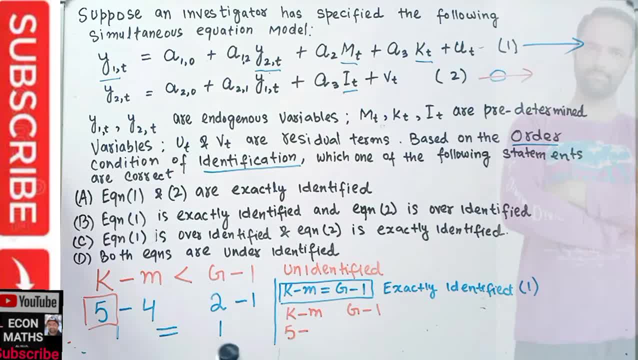 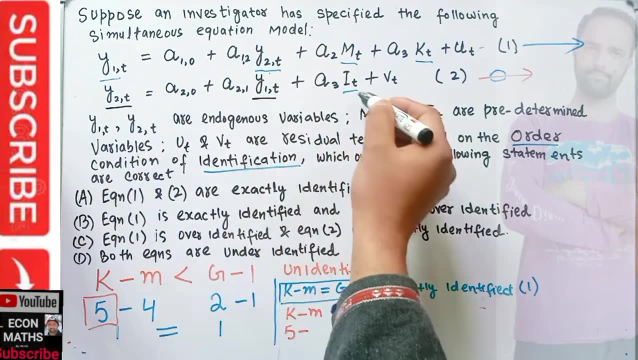 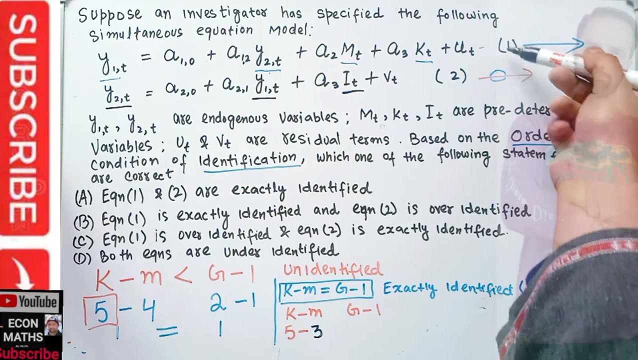 minus M. now we need to find out the M. that means the number of variables in this equation. okay, in the particular equation. so we have one variable, two variable, three variables. okay, so in the second equation, we have one, two, three variables. okay, so the value of M will be 3 and G, as we have seen. total number of. 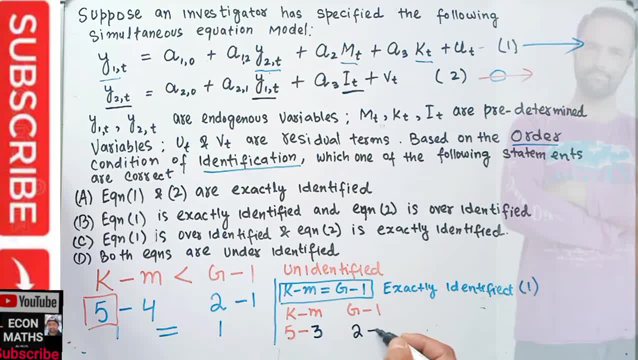 equations denotes G. so we have 2 minus 1. here we can see for you: minus 3 is 2 and 2 minus 1 is 1. here we can see 2 is greater than 1 and K minus M is greater than G minus 1. that means, if this is the case, we say that particular. 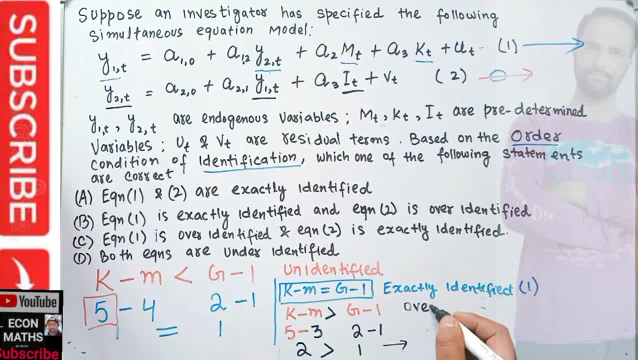 equation is over identified. okay, over over identified. so equation second is over and equation first- this very stuff here is exactly identified. so whether, let us see the options, equation 1 and 2 are exactly identified. no, this is not the case. okay, equation 1 is exactly identified. yes, we have k minus m is equal to g minus 1. this part is: 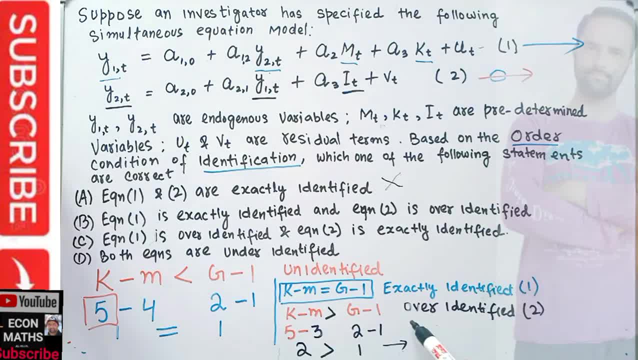 correct and equation 2 is our identified. yes, equation 2 is our identified, so this option should be correct. okay, so simple thing. what you need to do in the order condition and if we want to see whether a particular equation is identified or unidentified, what we need to do first, we need to see total number of variables in our model. okay, so let us say: 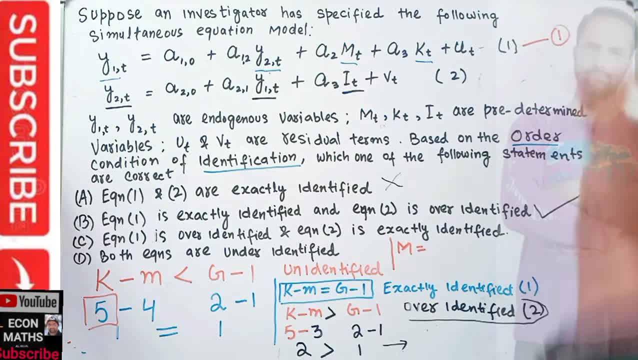 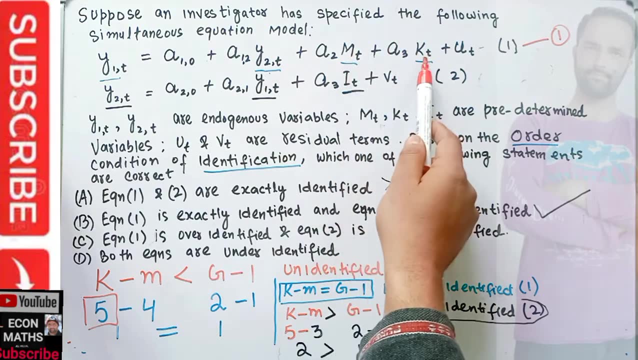 we are trying to find out whether first equation is identified or not identified. for that we need to find out the total variables in our model, whether they are endogenous or exogenous. so we have 1, 2, 3, 4 and 5- okay, we will not count this y1- t, because we have already calculated this. so total number: 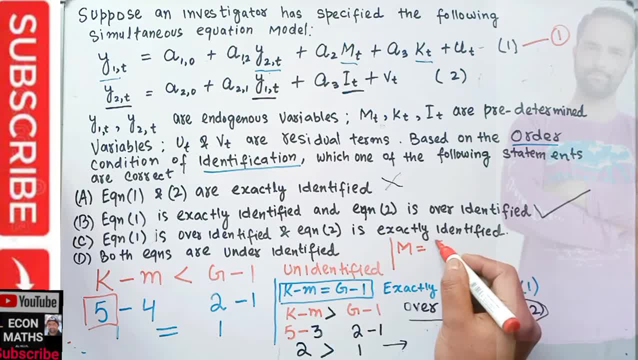 of equations- sorry, total number of variables is 5. after that we need to find out the number of variables in a particular equation. so in the first equation we have 1, 2, 3 and 4 variables. okay, and we also want to find out what is the value of g? what? 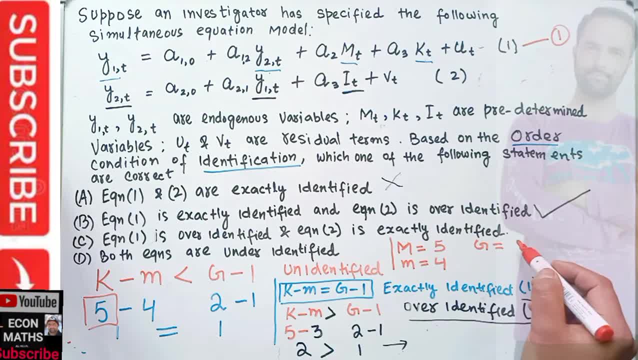 uh, how many equations we have. 1, 2. we have two equations. okay, then we use this very condition, that is, that is m minus m2 and what is the value of g I am gonna get? this is the values has that we use now. so here, we use now this condition to be the variable. we use the pl Warriors. 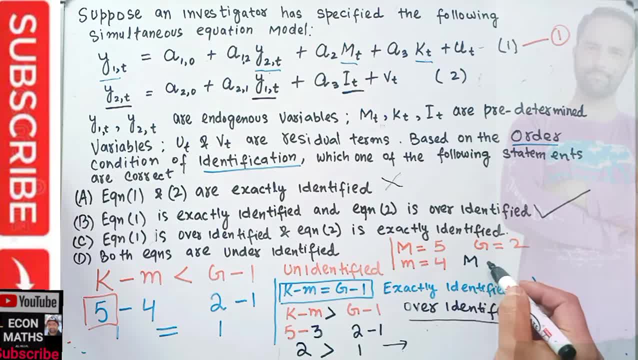 letters and I want to use the variator and what we actually want to ב here. see what's the value of bars, what's the value of and what's the value of l, which says that this something m minus m and g minus 1. okay, so m minus m means 5 minus 2. g minus m means 2, sorry, g minus 1.